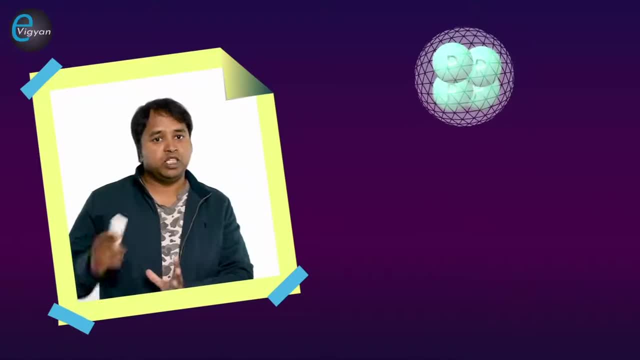 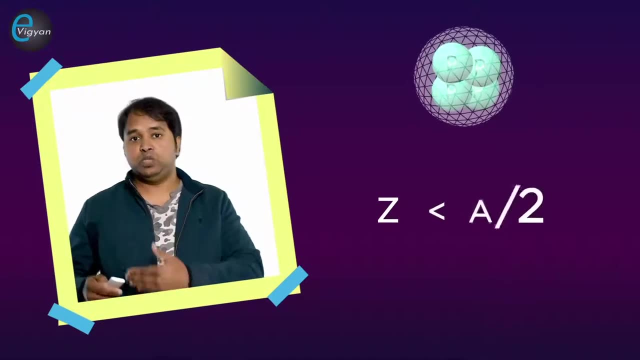 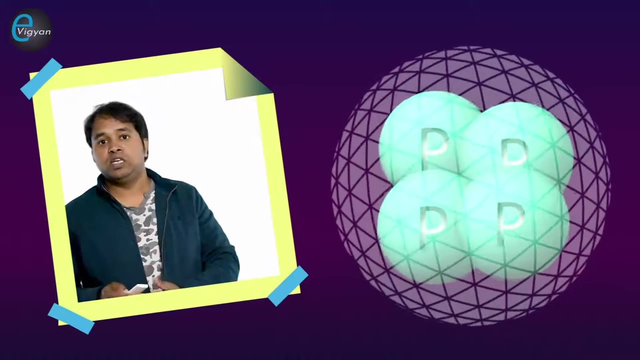 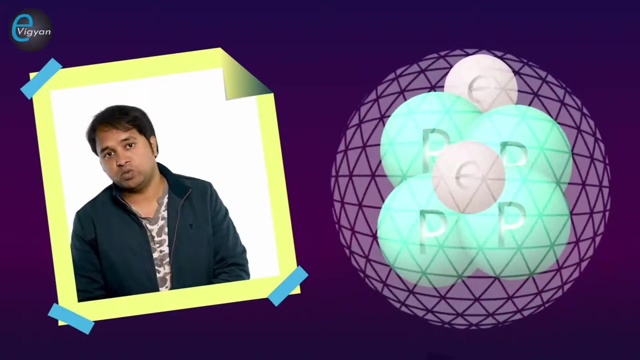 But it was already observed that, except for hydrogen, the nuclear charge G is found to be always less than A, usually less than A by 2.. To get around this difficulty, it was assumed early that, in addition to the protons, atomic nuclei contain just enough electrons to cancel the positive charge of the extra protons. 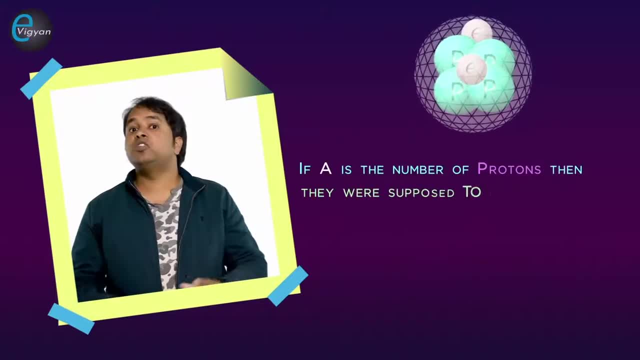 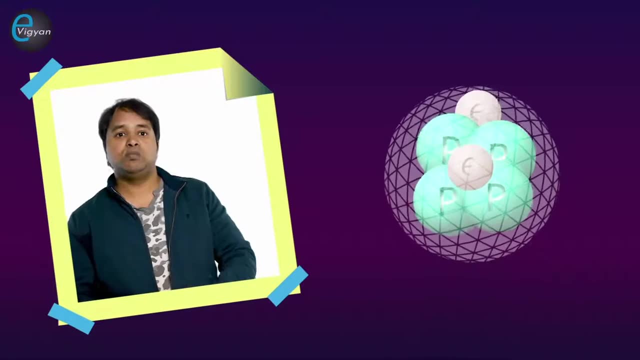 That is, if A is the number of protons, then they were supposed to contain A-G electrons. These electrons would contribute only a small amount to the mass of the nucleus, but together with the protons they would make the net charge G. 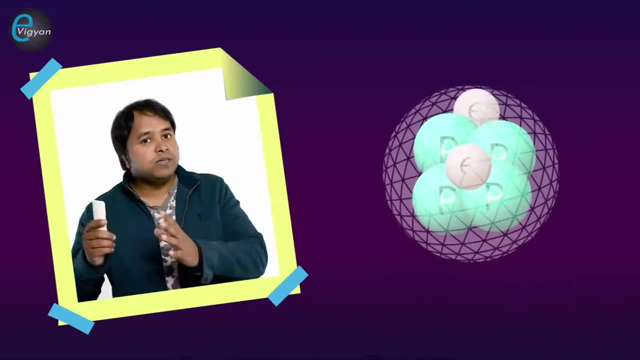 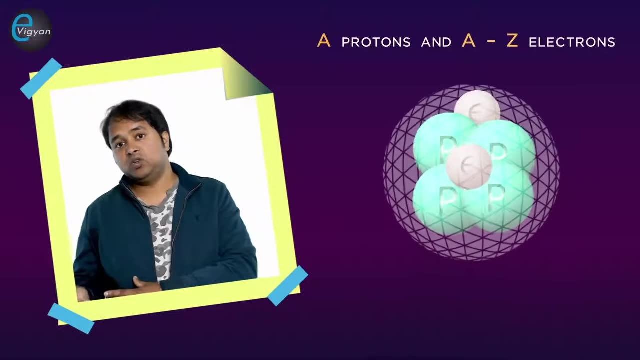 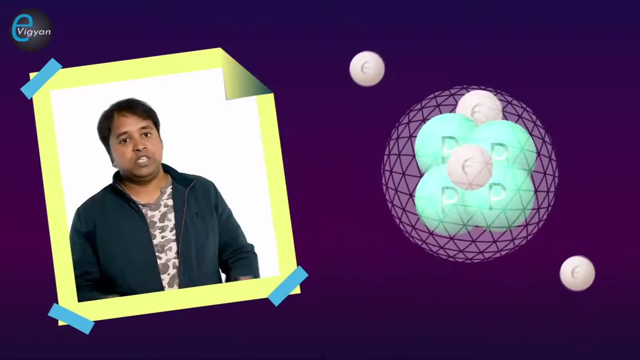 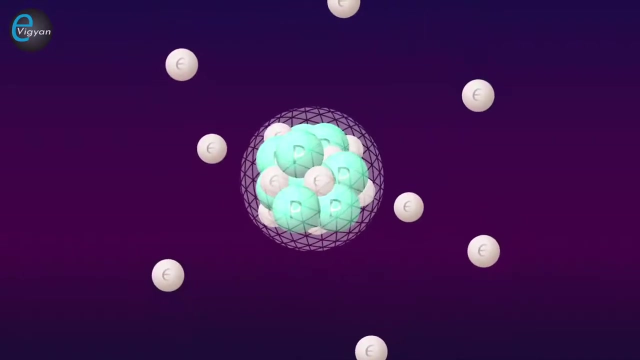 So it seemed plausible to consider the atom as consisting of nucleus made up of A protons and A-G electrons, with G additional electrons outside the nucleus to make the entire atom electrically neutral. For example, an oxygen atom would have a nucleus with 16 protons and 8 electrons, with 8 additional electrons outside the nucleus. 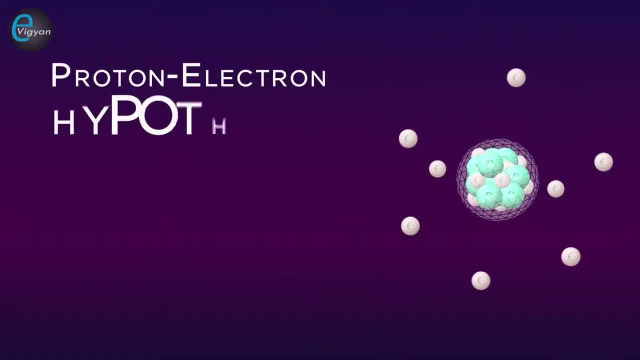 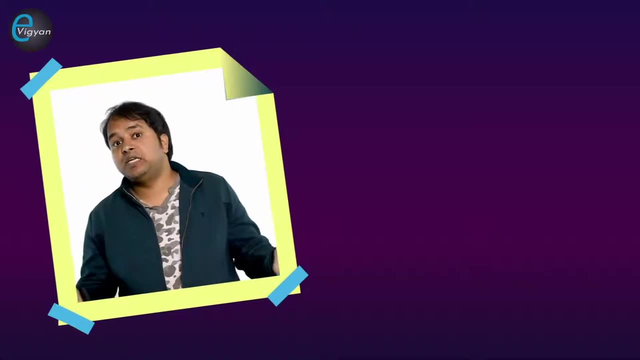 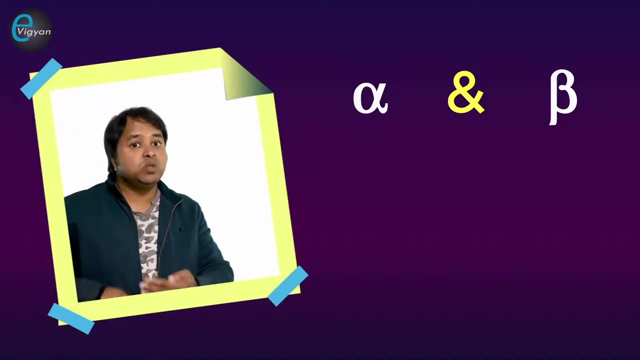 This model of the nucleus is known as the proton-electron matrix, The proton-electron hypothesis of nuclear composition. The proton-electron hypothesis seemed to be consistent with the emission of alpha and beta particles by atoms of radioactive substances. Since it was assumed that the nucleus contained electrons, the explanation of beta decay was no problem. 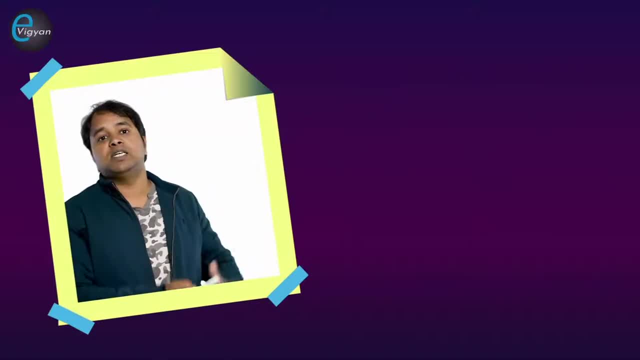 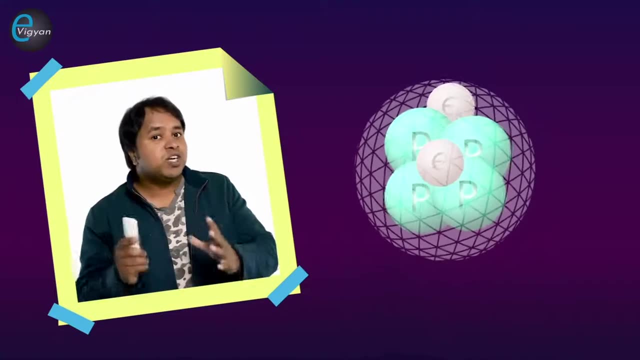 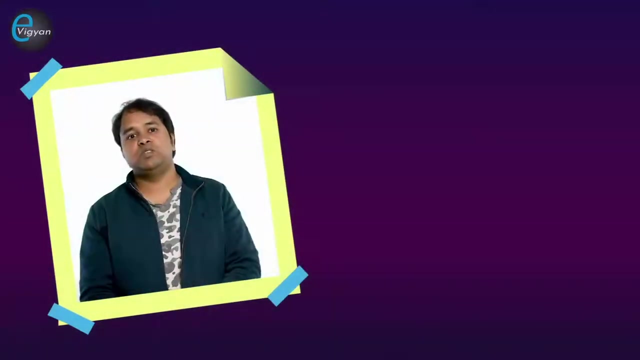 It also seemed reasonable that an alpha particle could be formed in the nucleus by the combination of 4 protons and 2 electrons. Although the proton-electron hypothesis was satisfactory in some respects, it led to serious difficulties and had to be given up. 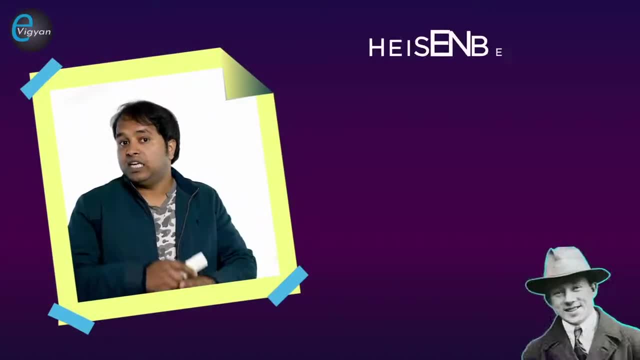 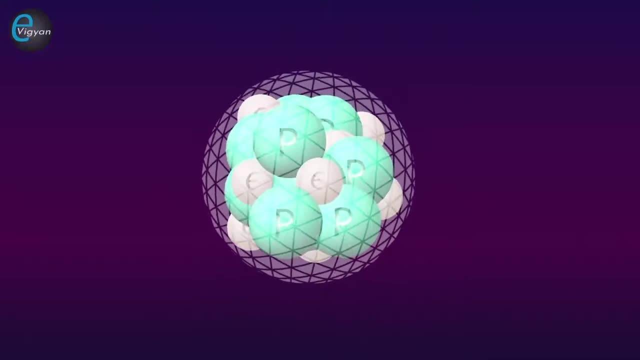 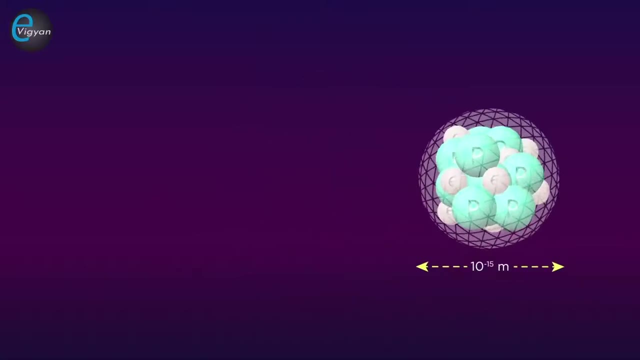 One of the most serious difficulties arose from the Heisenberg's uncertainty principle in quantum mechanics. If the electron has to be within the nucleus, then its de Broglie wavelength had to be of the order of the size of the nucleus. Since the size of a nucleus is in the order of 1 Fermi. 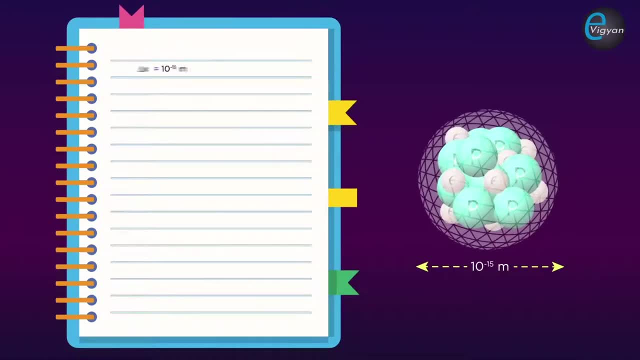 we can write the uncertainty in position of the electron as delta x equal to 10, raised to power minus 15 meter. Now if delta p is the uncertainty in momentum, then from the Heisenberg's uncertainty principle, delta p times delta x must be greater than equal to h cross upon 2.. 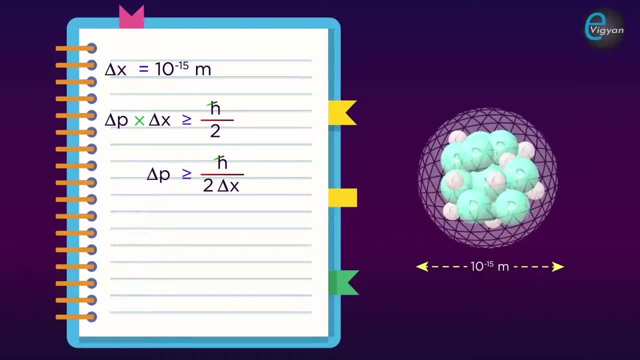 That is, delta p is greater than equal to h. cross upon 2 times delta x, which is equal to 197.46 MeV per c. Fermi upon 2 times 1 Fermi, which comes out to be 98.7 MeV per c. 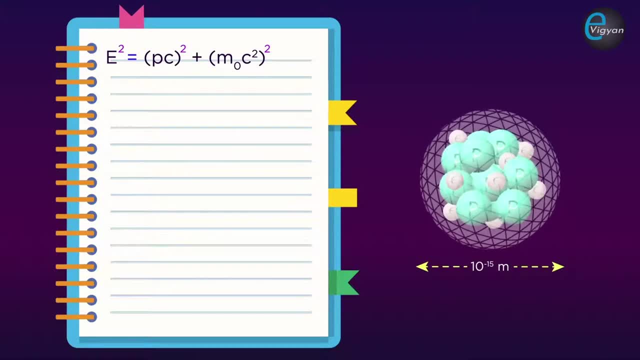 From the formula: e square is equal to p c square plus m naught c square, whole square. the energy of the electron corresponding to this uncertainty in momentum is e, equal to under root delta: p c square plus m naught c square, whole square. Here m naught is the rest mass of the electron. 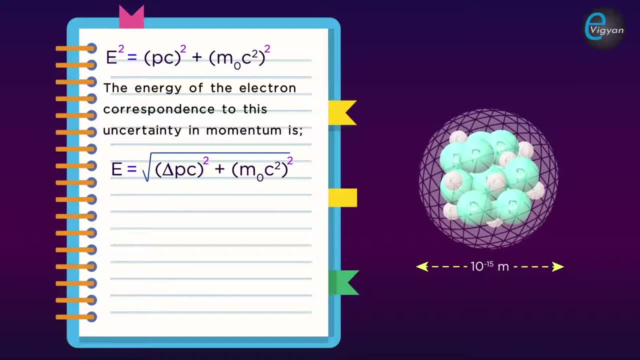 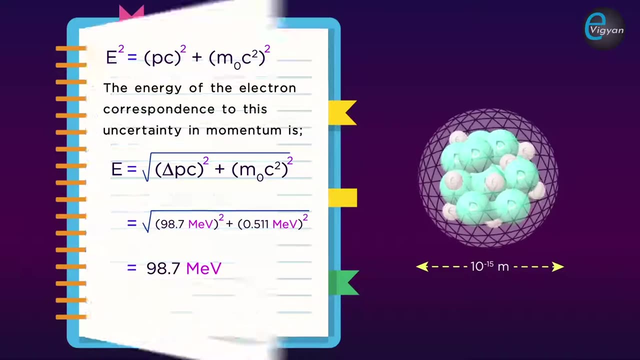 which is equal to 0.511 MeV per c square. Now we can write e equal to, under root, 98.7 MeV whole square, plus 0.511 MeV whole square, and which comes out to be 98.7 MeV. 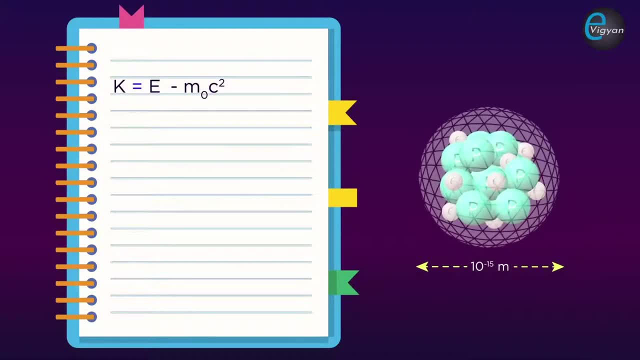 And the kinetic energy of the electron will be k equal to e minus m, naught c square, which is equal to 98.7 MeV minus 0.511 MeV, and that will be equal to 98.2 MeV. 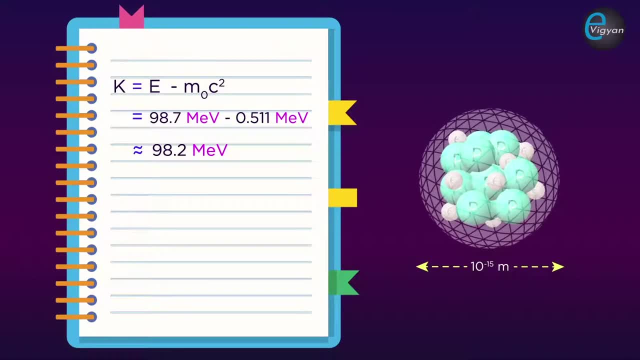 Now, if you calculate the speed of the electron with this kinetic energy, then it will be v, equal to under root 2 k by m naught, and which is equal to under root 2 times 98.2 MeV upon 0.511 MeV per c square. 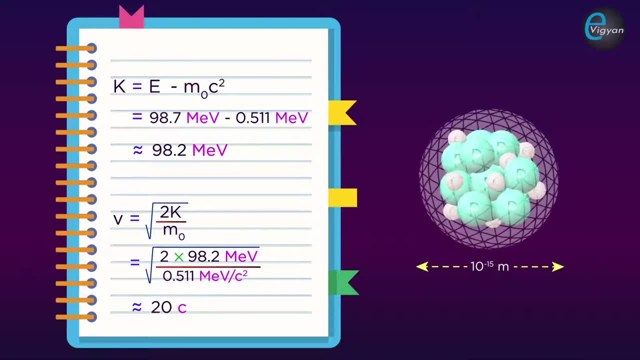 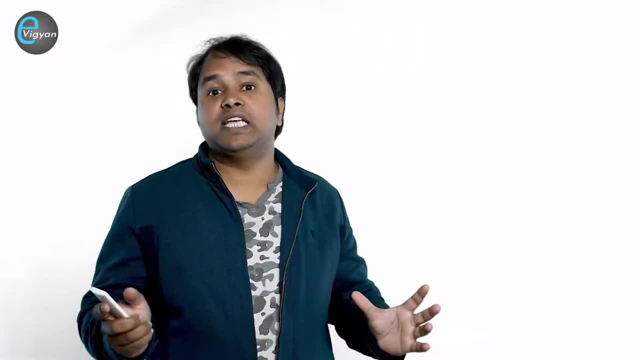 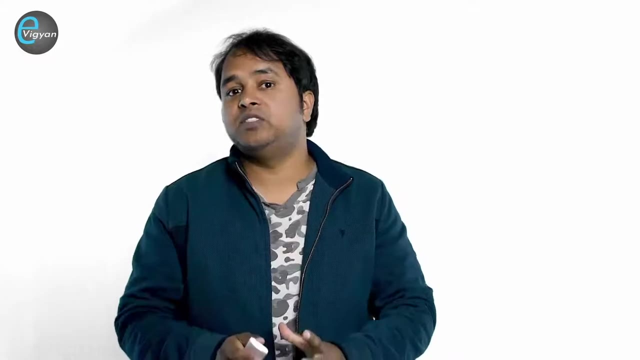 and that comes out to be 20 c, that is, 20 times the speed of light. So the confinement of an electron to a space as small as the nucleus would result in the circumstances that the electron's speed would be around 20 times the speed of light. 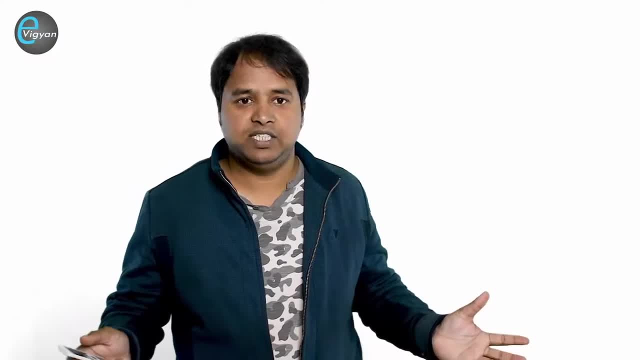 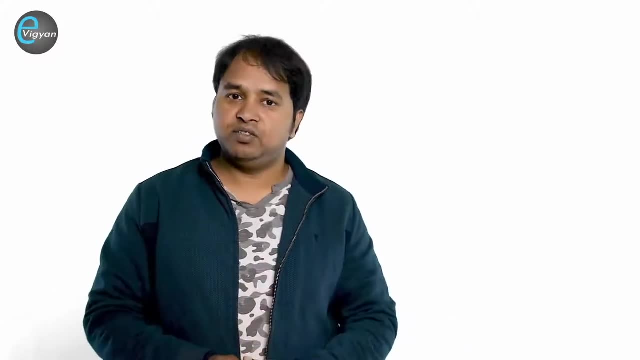 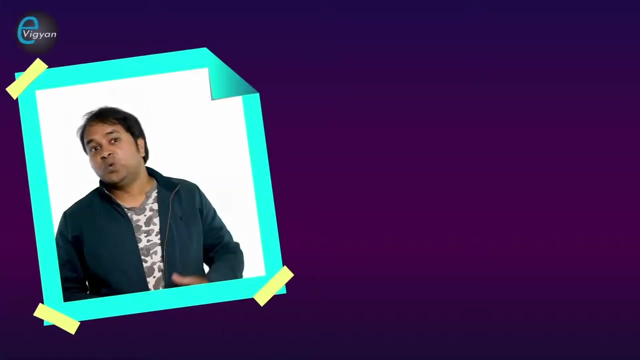 which is not possible according to the special theory of relativity. But how could scientists account for the circumstances that electrons cannot be confined within the nucleus, yet they emerge from the nucleus in beta decay. Well, there is a story behind this problem. One day, Heisenberg and his assistant were contemplating this problem. 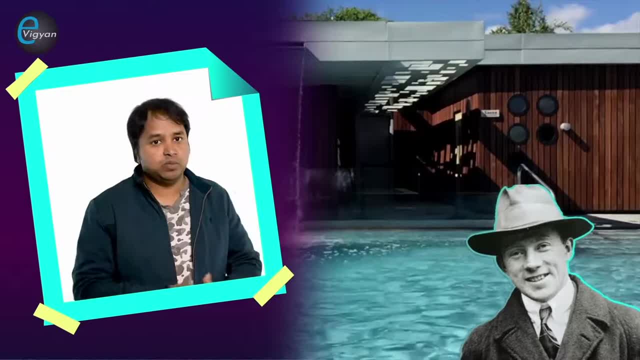 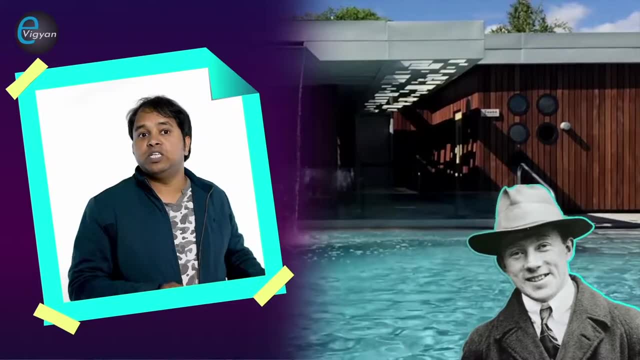 while sitting in a cafe across from a building hosting a swimming pool, Heisenberg suggested a possible approach to this problem. He told his assistant: you see people going into the building fully dressed and you can also see they are coming out fully dressed. 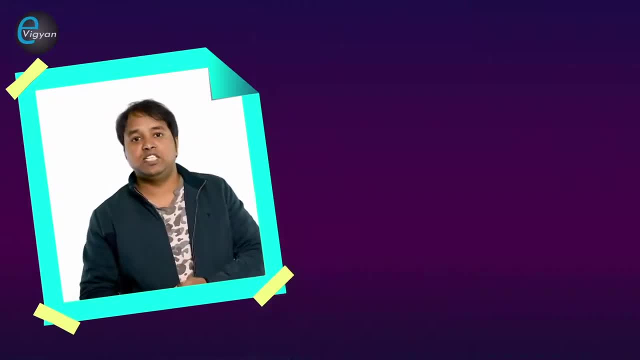 But how does that mean that they also swim fully dressed? He told his assistant: you see electrons coming out of the nucleus in beta decay and occasionally being captured by the nucleus. but that doesn't mean that electrons remain in the nucleus. Perhaps the electrons are created in the process of emission from the nucleus. 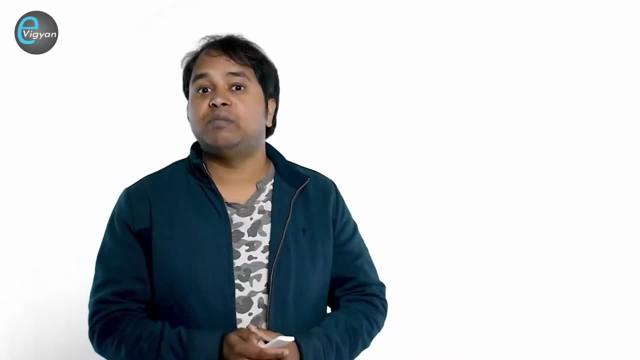 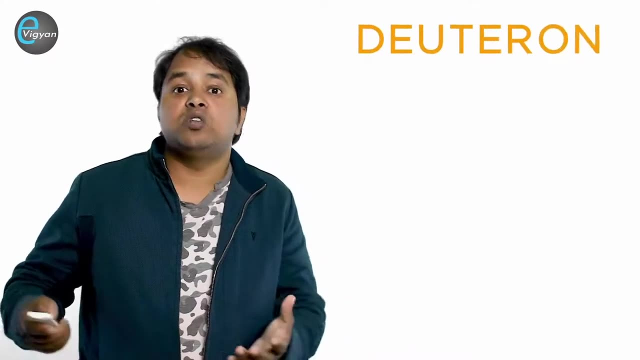 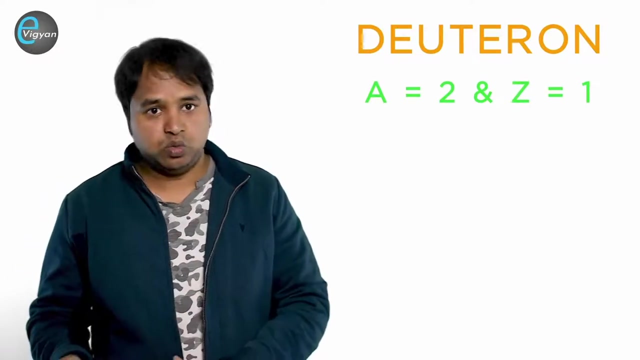 Later on, it was also observed that the proton-electron hypothesis violates the angular momentum coupling rule. Let's understand it by taking an example of deuteron. The deuteron is the nucleus of the isotope of hydrogen deuterium. The deuterium has A equal to 2 and G equal to 1.. 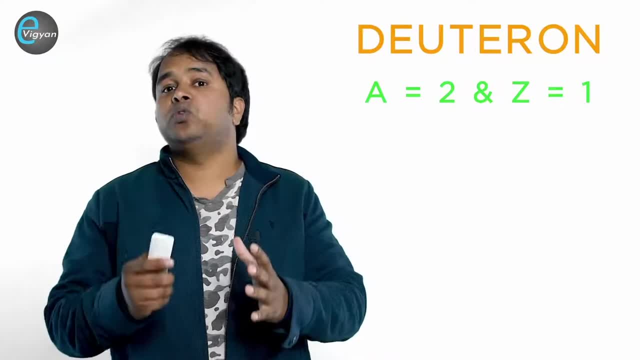 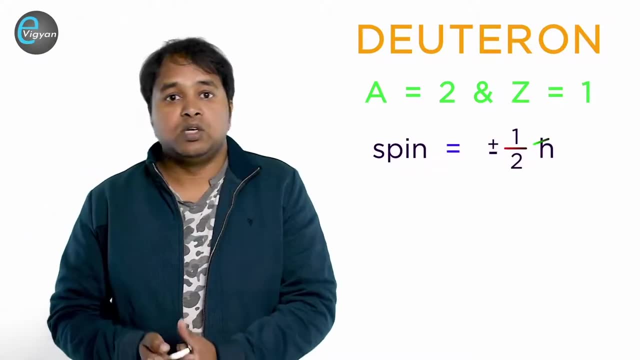 So from the proton-electron hypothesis there would be two protons and one electron, Since proton and electron both have a spin equal to plus minus half h cross, which can simply be written as plus minus half, because in natural unit h cross equal to 1.. 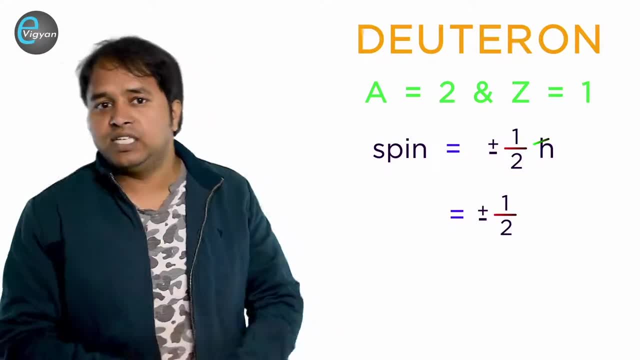 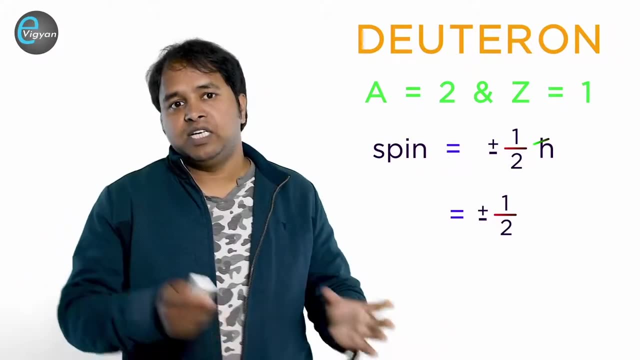 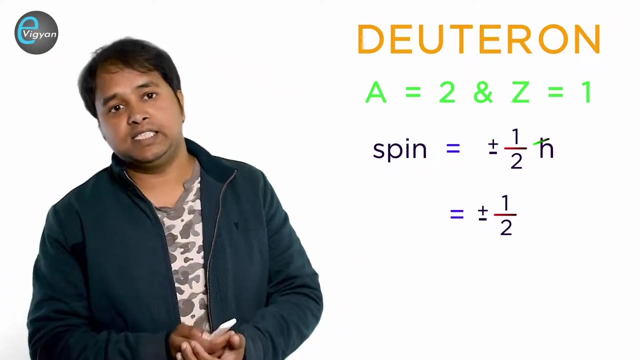 If you want more information about natural unit then you can click here and watch the video of natural units. So for proton and electron we have a spin equal to plus minus half. Here plus sign is for the spin along plus z-axis and minus sign is for the spin along minus z-axis. 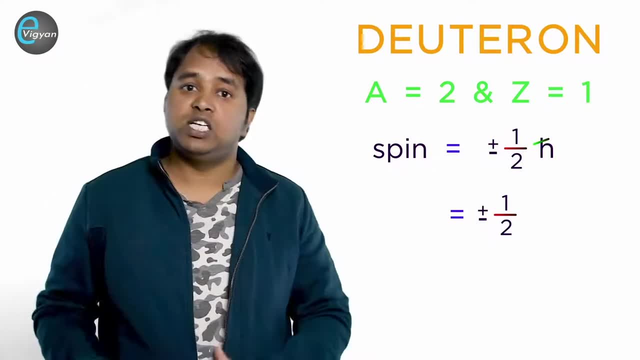 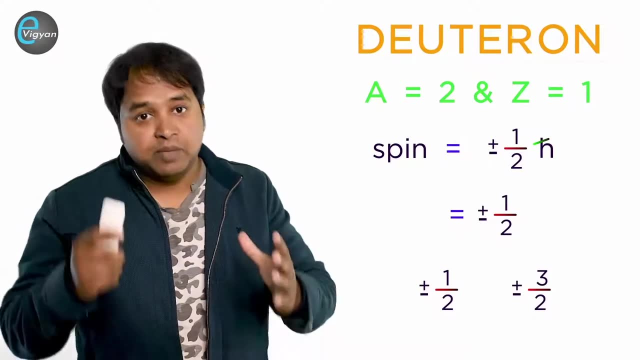 When you add the spin vectors of two protons and one electron, then the possible spins of deuteron would be either plus minus half or plus minus 3 by 2.. But the measured grand state spin of deuteron is calculated as plus 1.. 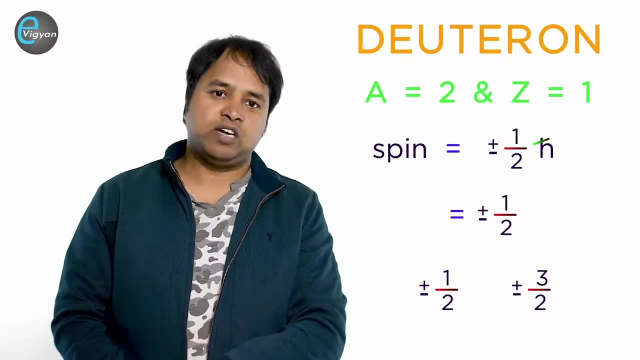 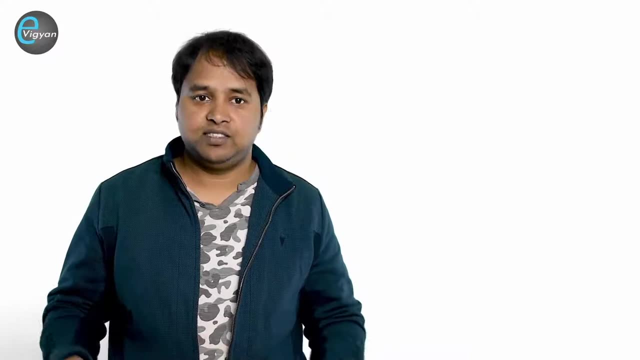 And it is also a major problem for the proton-electron hypothesis. Now let's prove the proton-electron hypothesis wrong by calculating the magnetic moment value of the nucleus. The magnetic moment of electron is equal to E, h cross by 2 Me, where Me is the mass of the electron. 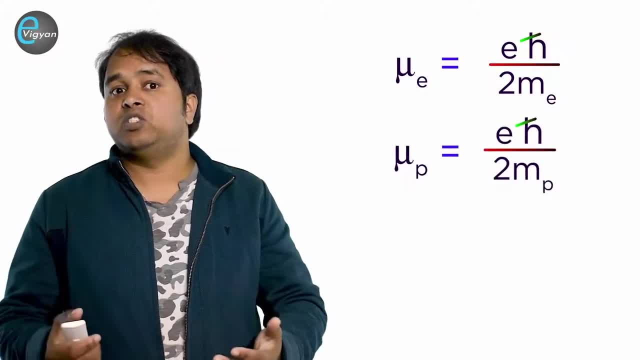 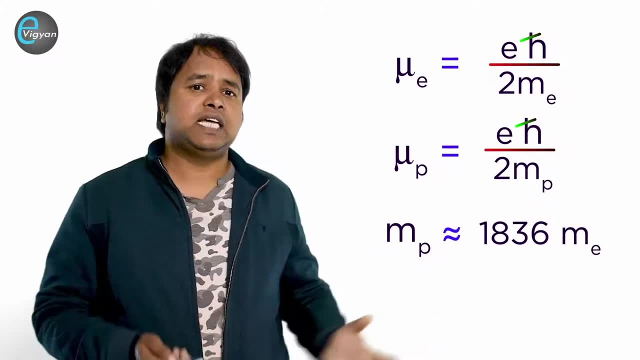 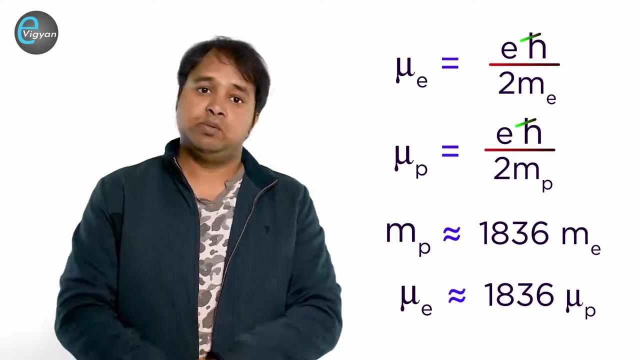 and the magnetic moment of the proton is equal to E, h cross by 2 Mp, where Mp is the mass of the proton. Since the mass of the proton is almost 1836 times the mass of the electron, so the magnetic moment of the electron would be almost 1836 times the magnetic moment of the proton. 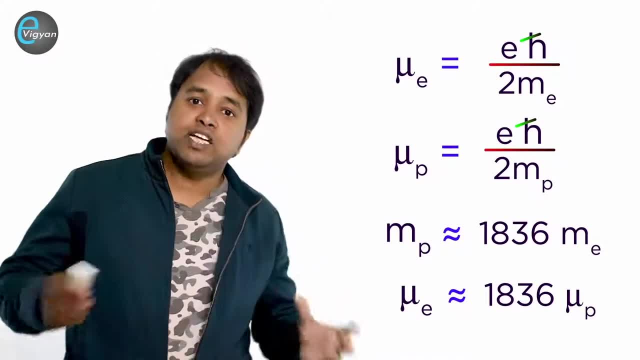 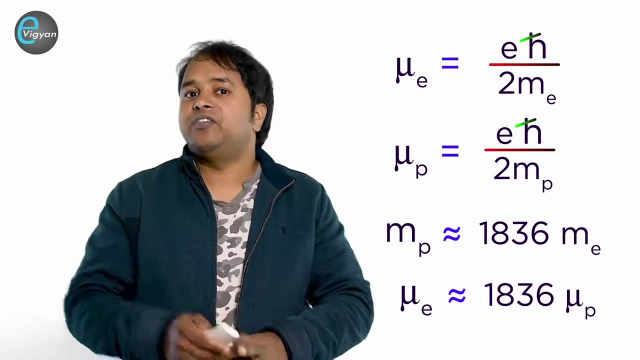 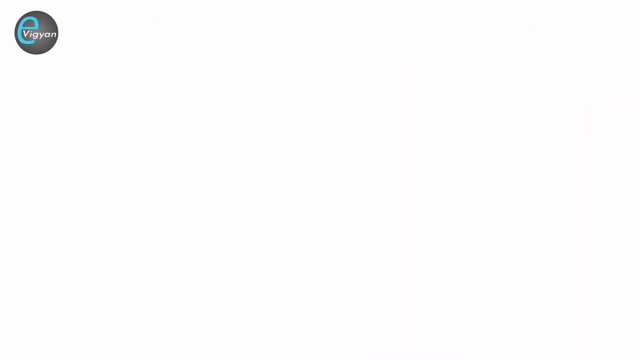 Now, if an electron would exist in the nucleus, then the nuclear magnetic moment would be of the order of magnetic moment of the electron. but the measured magnetic moment of the nuclear are very much less than the magnetic moment of the electron. thus the electron cannot reside inside the nucleus. 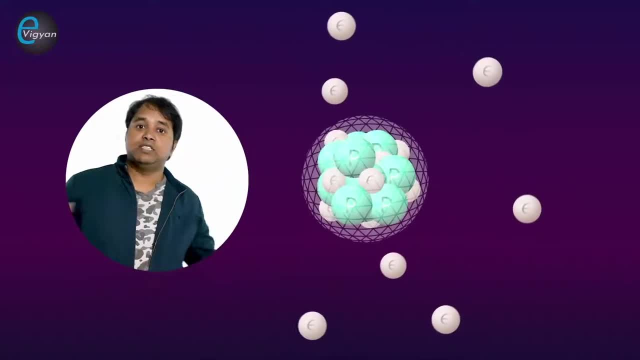 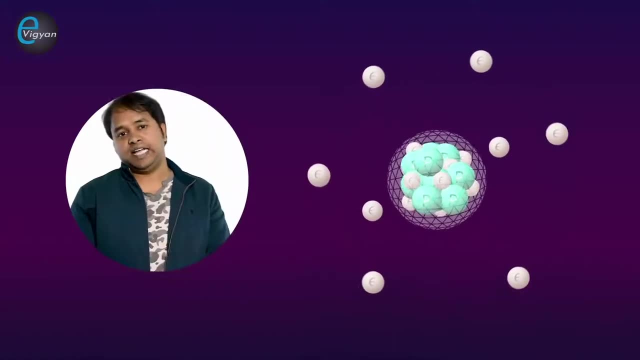 Also the presence of some electrons in the nucleus and rest as peripheral around the nucleus, exhibit the dual role of electrons in an atomic structure, which is difficult to understand. So this is all about the problems behind the proton-electron hypothesis of nuclear compositions. 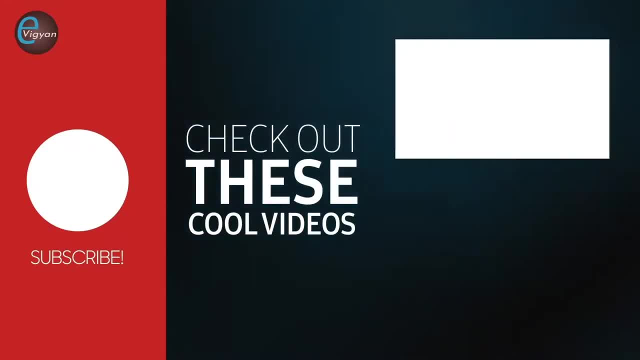 Thank you so much for watching this video. See you in the next video. 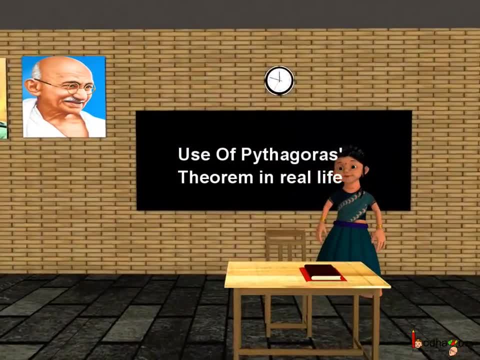 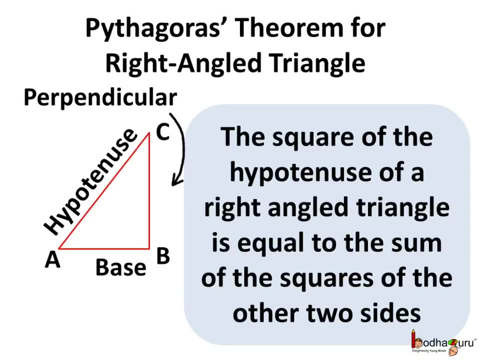 Good morning children. Today we shall learn about the use of Pythagoras theorem in real life. We already know what is Pythagoras theorem and it explains the relation between the sides of a right angled triangle. The Pythagoras theorem says the square of the hypotenuse of a right 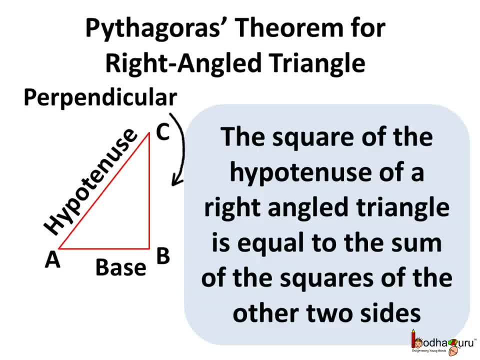 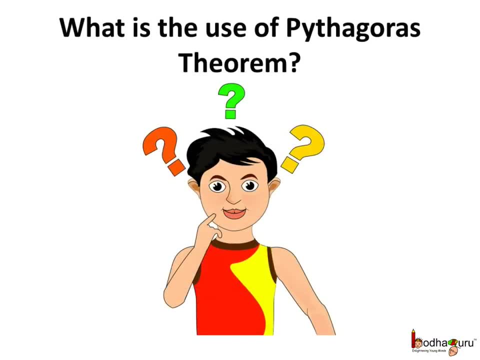 angled triangle is equal to the sum of the squares of the other two sides. So according to it, square of the hypotenuse is equal to square of the base plus square of the perpendicular. What are the uses of Pythagoras theorem in real life? Let us see. Pythagoras theorem is very. 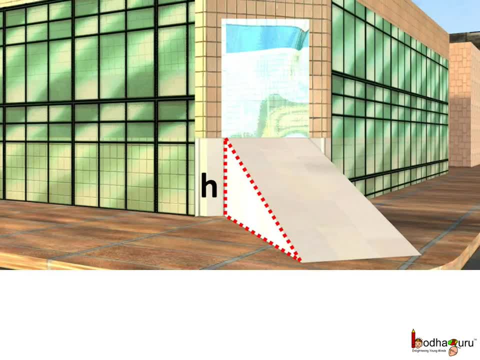 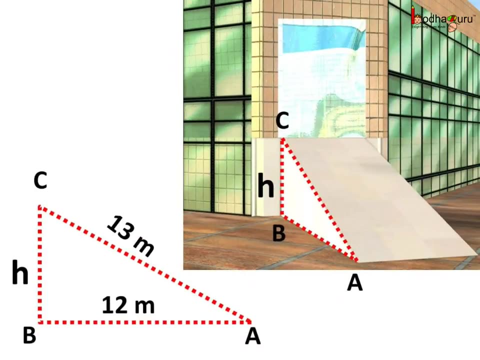 useful in real life. For example, Now we want to measure the height of the plane ie h in the picture. Look at the plane. It is forming a right angled triangle with the ground. Let us name this triangle as ABC. The length of the slanting plane is 13 meter and the distance between the starting